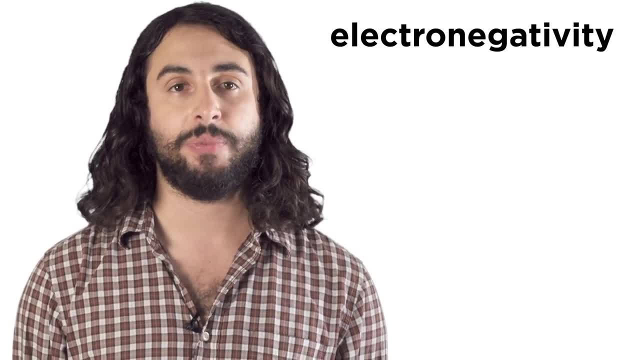 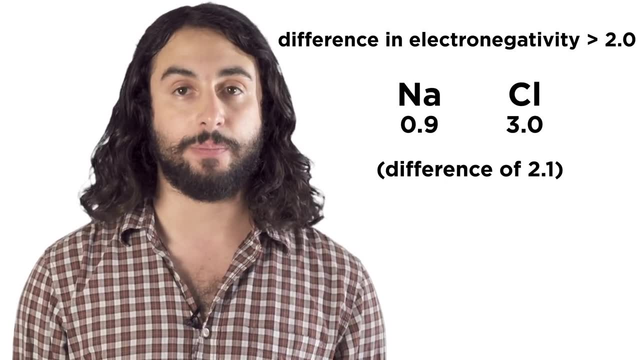 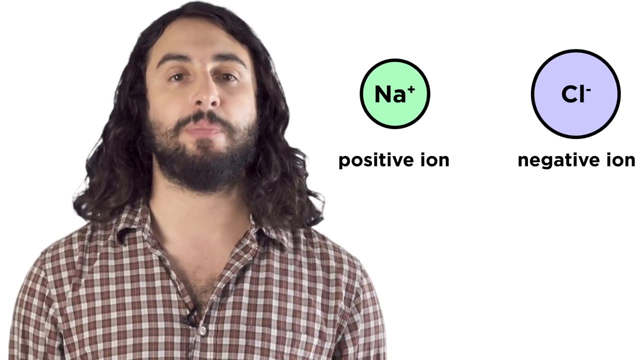 electronegativity between the two atoms participating in the bond. if the difference is more than about two, like with sodium and chlorine, chlorine will steal an electron from sodium. chlorine really wants another electron, sodium really wants to get rid of one. so everybody wins. the result is a 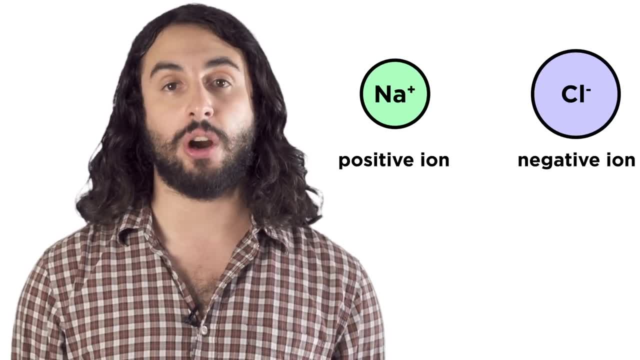 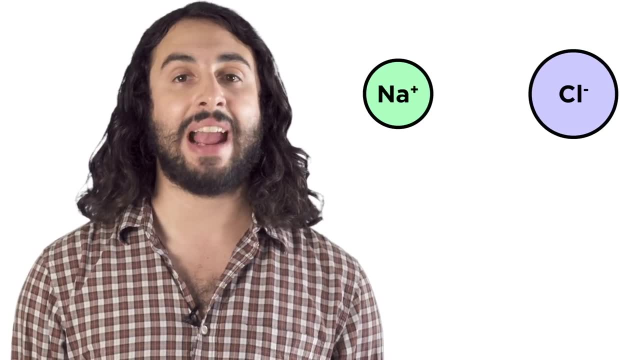 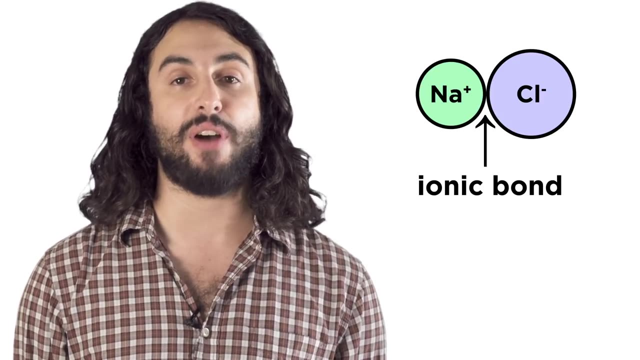 positively charged sodium ion and a negatively charged chloride ion. particles of opposite charge have an electrostatic attraction, so these two ions hang out together by forming an ionic bond. this is a very strong attraction because it is happening between ions that have a formal charge. 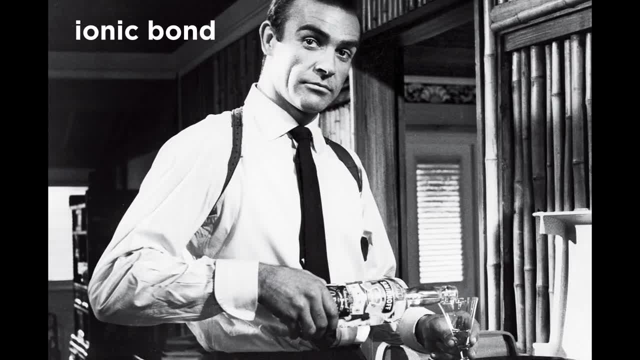 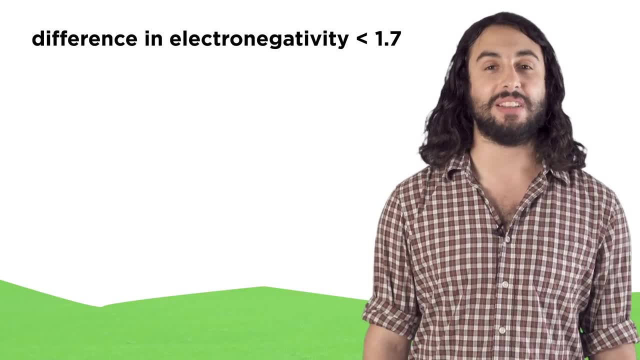 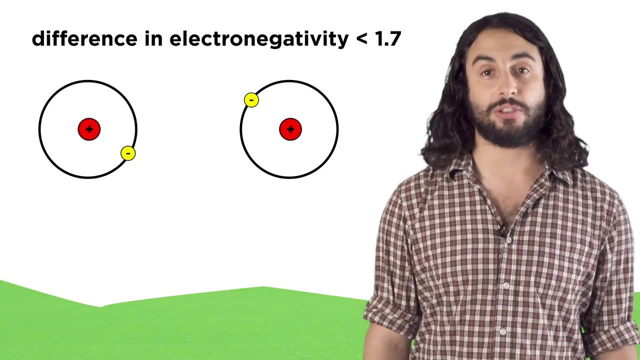 bond. ionic bond bond: electrons taken, not shared. speaking of shared electrons, if the difference in electronegativity between the two atoms is less than about 1.7, no electrons are stolen, but instead the two atoms share two electrons: the electron. 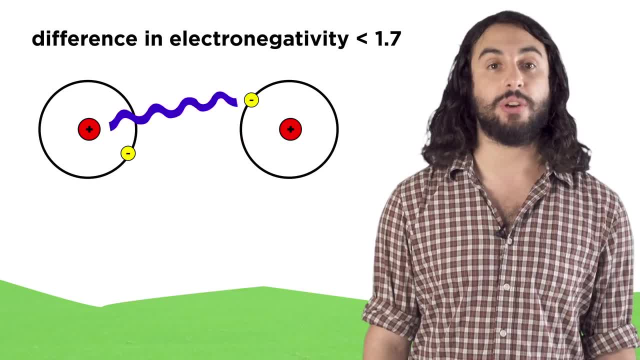 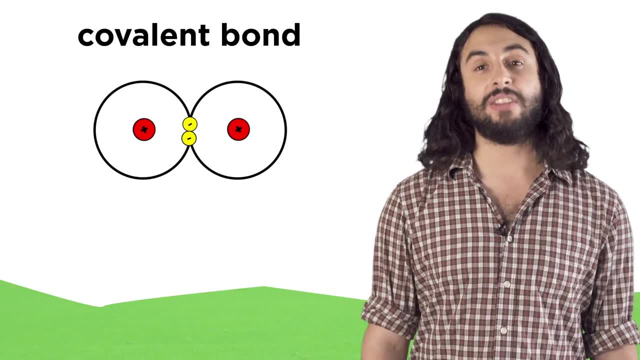 from this atom feels the attraction from the other nucleus and so does the electron from this atom. so the atoms share the two electrons to form a covalent bond. covalent bonds can be polar or nonpolar if the electronegativity difference between the atoms is not high enough to cause. 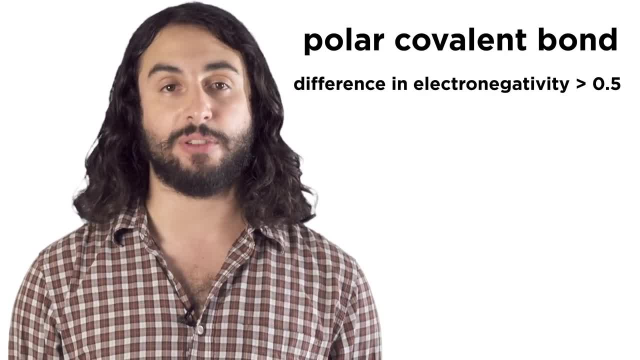 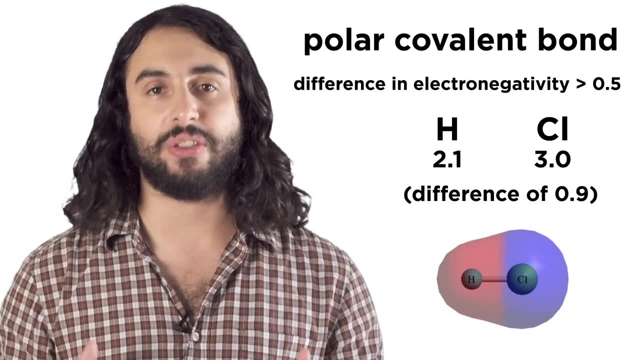 ionization, but is at least more than 0.5 or so. like with hydrogen and chlorine, instead of completely stealing the electron, the chlorine will just sort of hog the electrons in the resulting covalent bond, the more electronegative 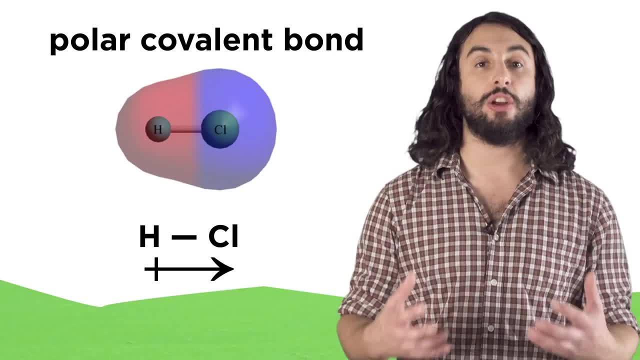 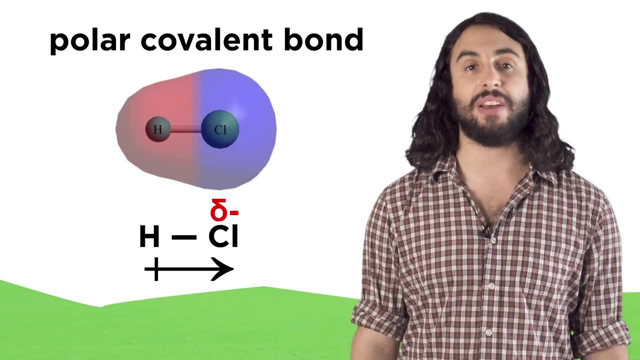 atom in a polar covalent bond pulls the electron density towards itself and, as a result of the slight electron excess, we call this atom partially negative, denoted by the symbol delta minus. the atom whose electron is getting pulled away is slightly electron. 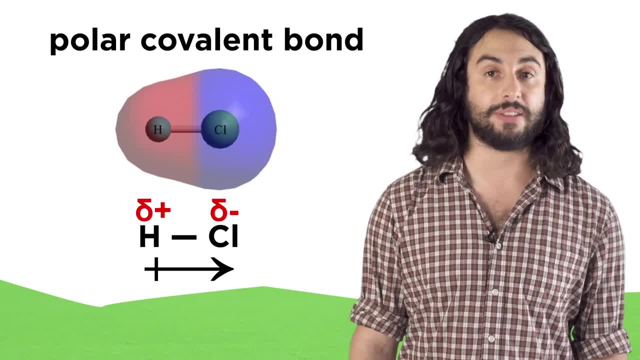 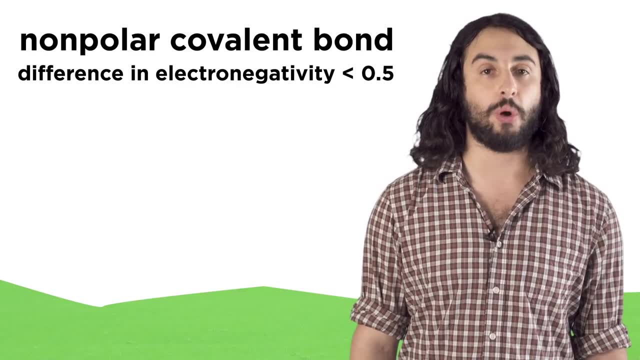 deficient and therefore partially positive or delta plus. if the electronegativity difference is less than 0.5,, the covalent bond is said to be nonpolar. in a nonpolar covalent bond, the electrons are shared more or less. 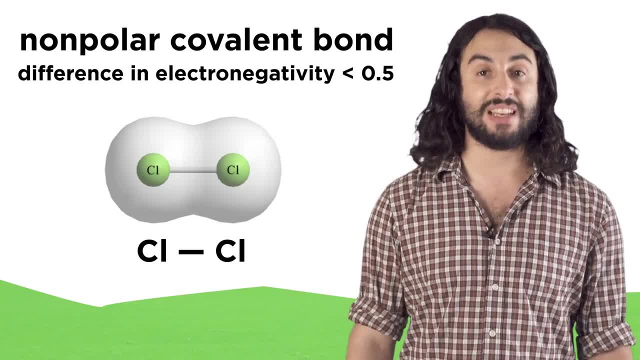 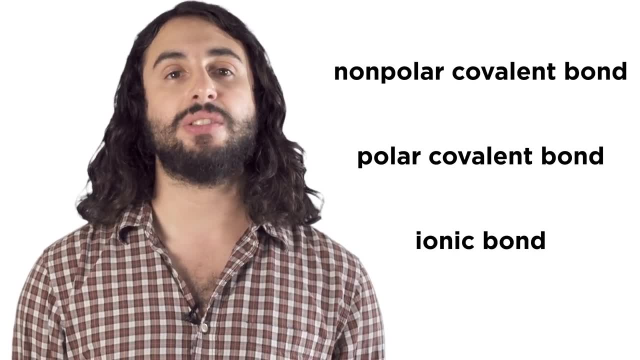 evenly, or in the case of two atoms of the same element, precisely evenly, the atoms will have no partial charges at all, other than strange phenomena like metallic bonding, the main ways atoms bind to one another. remember that you can predict the type.